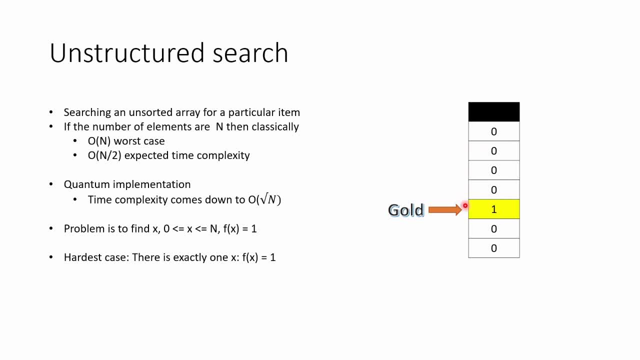 0, f of 2, it would go and say 0, f of 4, if I give 4 it will say f of 4 is 1.. So when I get, f of 4 is equal to one, I know. fourth location is where we have the gold. So we are trying to find the Gold. 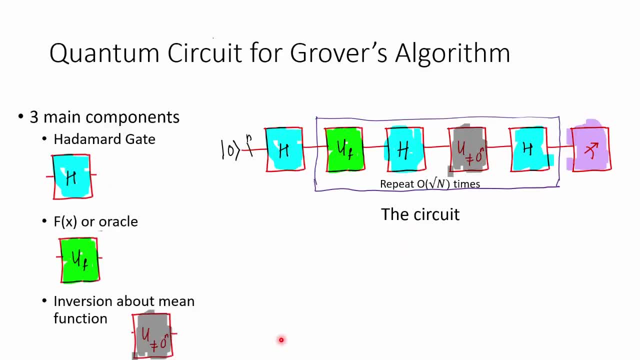 //point 1//, // quilt humorcoil //, // arbello//, // Dragon Explorer // is the quantum circuit for Grover's algorithm. so I'm not going to explain what Grover's algorithm is, how this Grover's algorithm actually works. if you need me to do that, I will do another video on that. please put your comments. 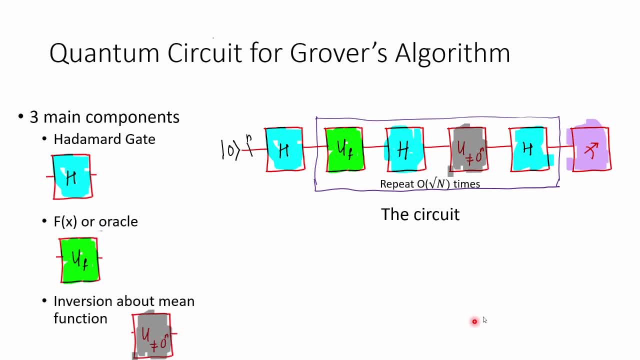 on the comment section. I will do that, but technically, you know, imagine there is a lot of magic and at the end of it we can implement Grover's algorithm. and this is how the Grover's algorithm will look. it has a series of gates, so it. 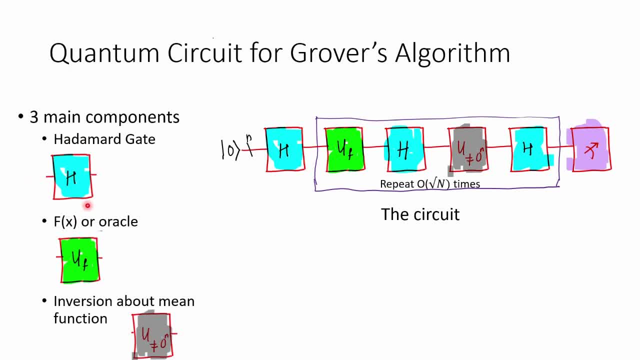 starts with three main components. it has a Hadamard gate, an f of X or the oracle and inversion about mean function. this is the three different gates. I will go and specifically explain the implementation of each of them, but what it looks like is like this: you have an input which is all zeros, n inputs, n bit. 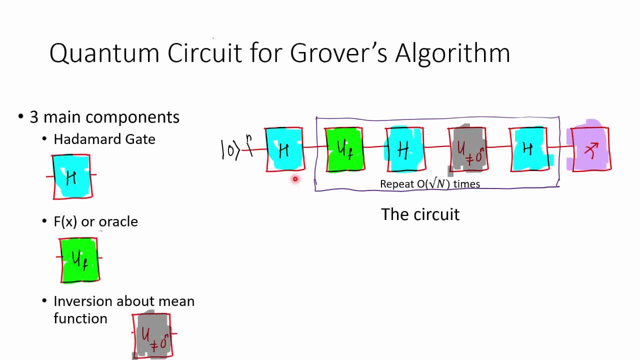 n zeros and it will apply to Hadamard gate. what this does is up. once this Hadamard gate is applied to all the zeros, at this point the magic of quantum mechanics happen. the value of all the bits here is a superposition state, which means the value of bits there represent all the 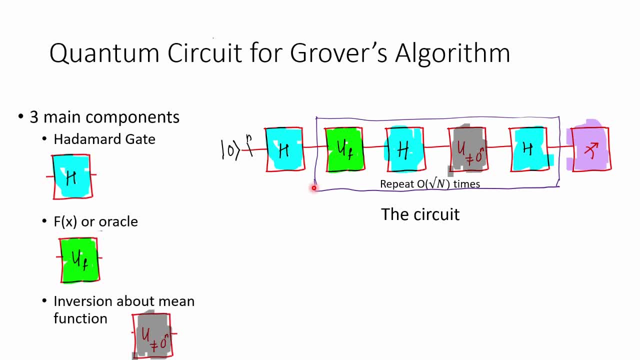 possible numbers. so it will be 0 0 0, 0, 0 0, 1 0, 1 0 0 0, 1 1 1 0 0, etc. etc. it is not just one particular input. so all the different inputs are given at the same time to the. 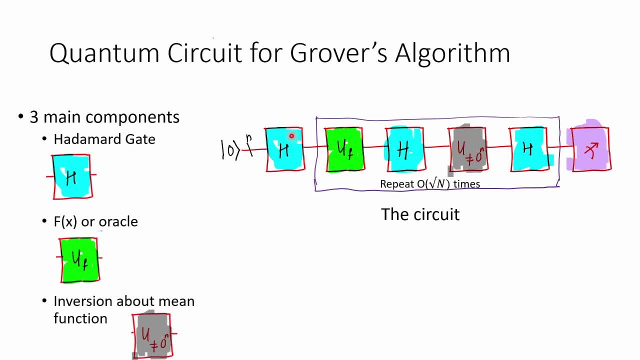 quantum circuit. so that is what Hadamard gate does. okay, I'm deviating from the point. so you have an Hadamard gate, then your u of f, u of f is basically the f of X function oracle. so, as I said earlier, if you give 4 here will give a 1 as 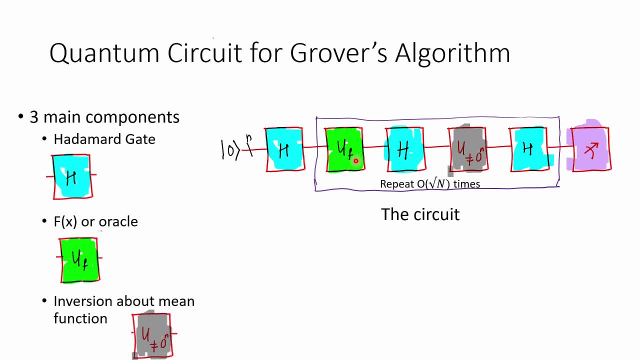 output everything else, it will be 0 right. so that is the u of f. so you, this u of f is a black box for you and you need to find what is the secret within this u of f. and then again another Hadamard gate, and then there is a mean function, mean. 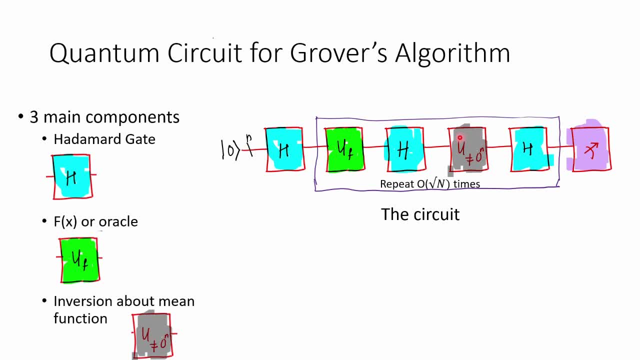 inversion right. we will see what that is, how that function looks like, how to implement that, and then another Hadamard and this part which I have put a box. this will be repeated root n times. so that is why this is one step. after this one step, I will do the same step root n times after root n times. I will just 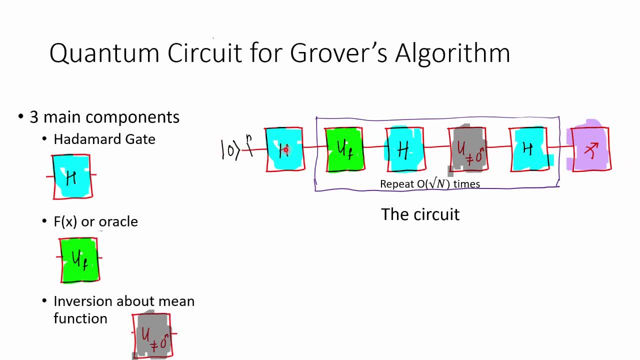 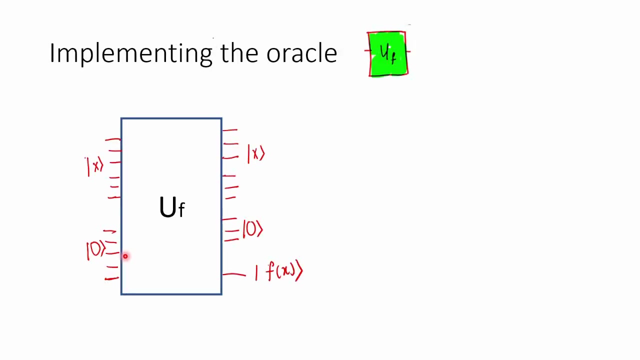 measure the value of the output bits, so the all the input bits. I will look what the values are and the claim is that, with a very high probability, I can recover the number where, uh, the gold is located. okay, now let us look at how to implement each of these components. so this is how implementing the Oracle looks like. 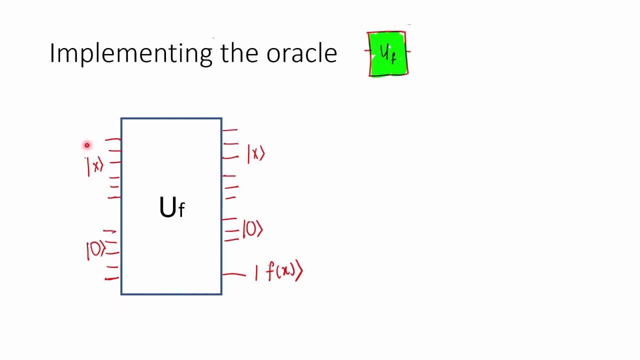 so Oracle u of f will look something like this: it have a number of bits which take the input X, a, which give the answer f of X. so it's either zero or one, based on what input comes here. there will be some extra zero bits here. uh, this will help to create the circuit u of f. you know every program. 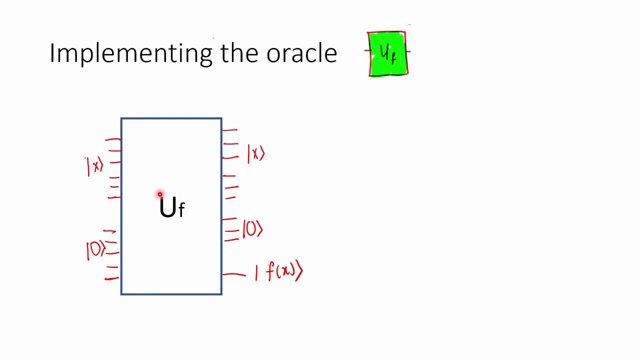 or every algorithm or pseudocode at the end get converted into a circuit in classical computer, just like that. it will end up converted into a quantum circuit here and that is one output here. then, similar to all the zeros here, there will be a lot of zeros here. 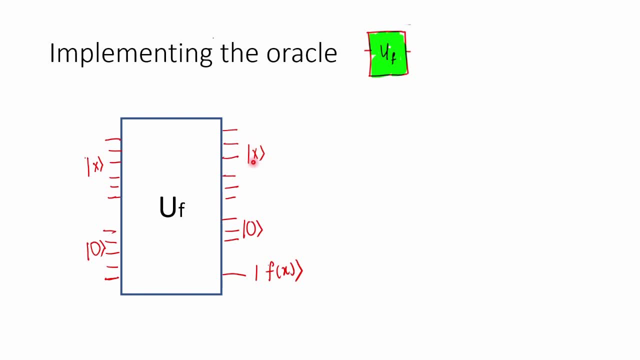 and all the X bits that come here will also be outputted here as X. so if you give zero, zero, zero, zero, here will be zero, zero, zero, zero, zero. you give f of zero, zero, zero, zero and a lot of zeros. that is what u of f looks like. we'll see in a minute how this is implemented. 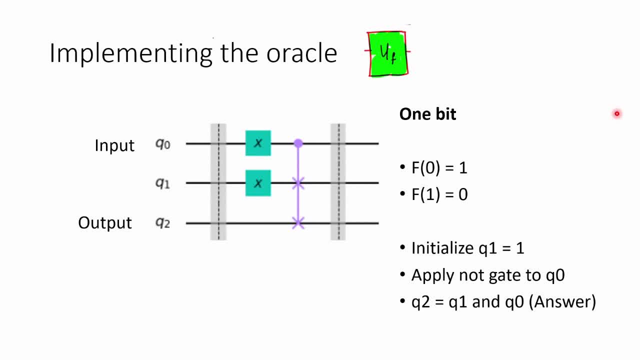 so let us see how we can implement the Oracle. start with one bit. so one bit basically means there are only two elements in the array, because right, so f of zero can be one or f of one can be one. for the time being, let us take f of zero, equal. 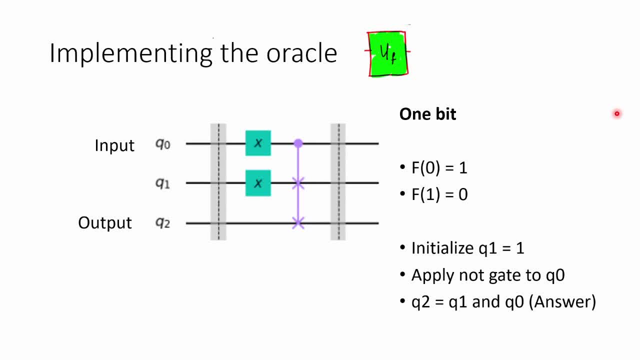 to one. so the, the gold mine is at the location- zero, right. so we have a initial input of q0 and then we have another qubit, q1, right? let us assume that this is where the answer is and let us assume that the answer answer is initially one. so we'll give zero here and this. 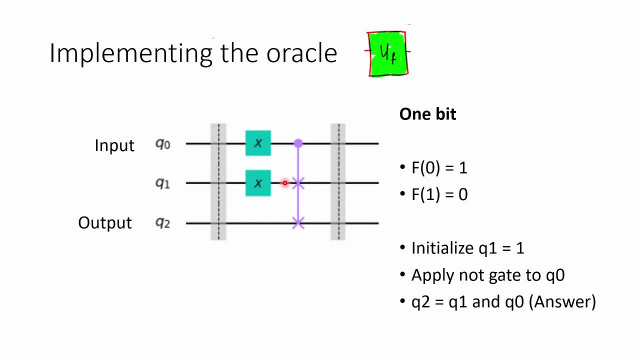 will convert the answer to one. so this is one. so right now, what we are assuming is that the answer is one and based on this qubit, we will change the answer right. so if this qubit is zero, then this part, you know, I apply an X over here and X becomes one. so this is the. you know how. 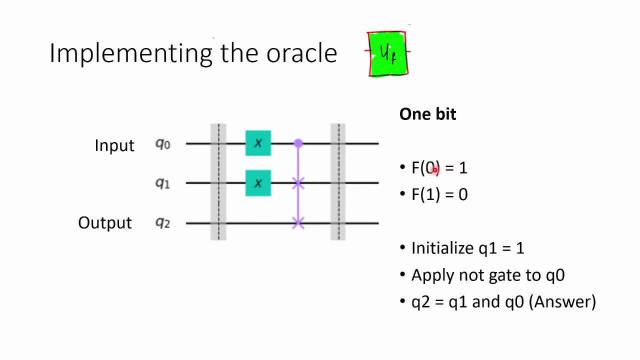 the function look like. I know that f of 0 is where the gold is, so if it is uh, uh, so I put comes 1 here. okay, and when this is 1, this should not change. when this is 0, this should change to 0. so basically, I need to do an AND of q0 and q1 to get. 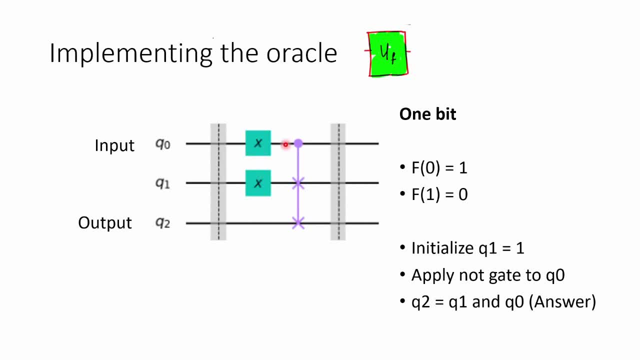 the answer right. so it AND q0 and q1 and store the result in q2. okay, so for that we use this quantum gate called C swap, which does something very similar to AND gate. so it takes q0 and q1, AND it, and the result of q0 and q1 will be in q2. 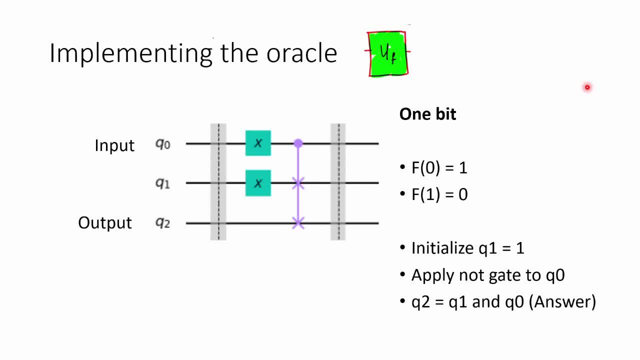 so do you find any problem with this circuit? it looks pretty okay. it has one input bit, q0, and according to that q0, it finds the answer in the output bit, q2. everything looks fine, correct. but there is one caveat: Q1 and Q2 are the same, but they are different. 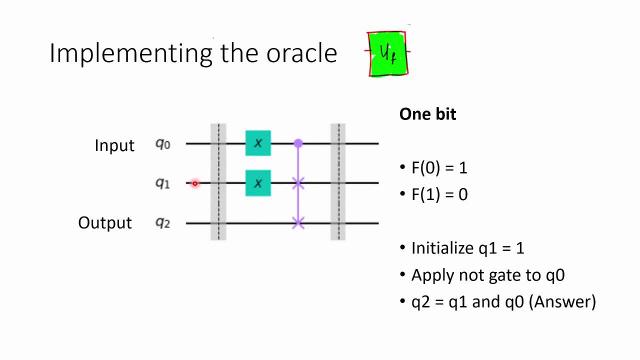 q0 and q1, their states, initial state is completely changed at the output bits. because of these circuits inside, because of these gates in the circuits inside which act upon q0 and q1, the value of q0 and q1 over here is not the same as it is. 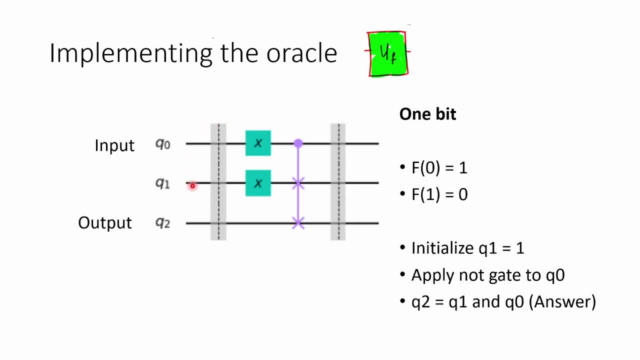 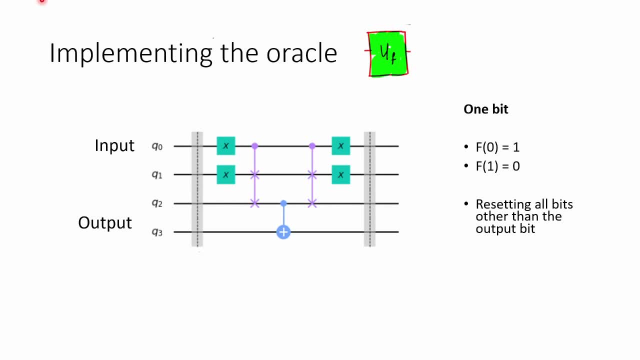 here in the input. we need to find a way to reset this. this is a very easy way to do this. this is a very easy way to do this. most, all, almost all- quantum gates are reversible. for instance, a NOT gate is the reverse of itself. so if you apply a NOT gate, another NOT gate will nullify. 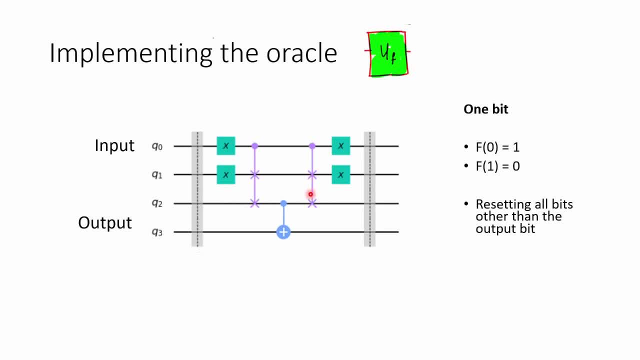 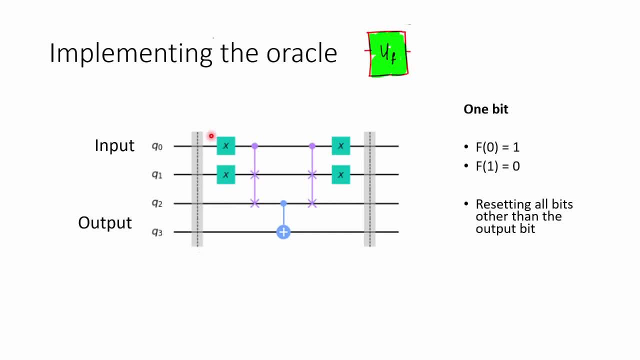 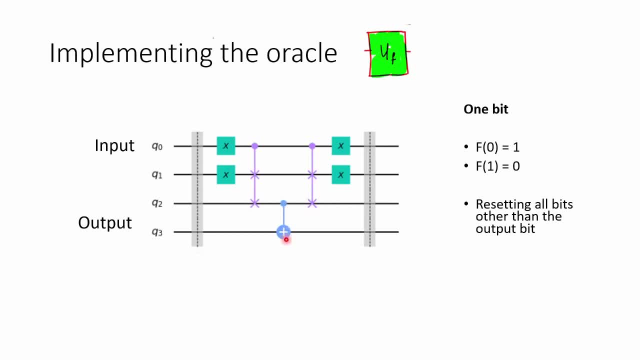 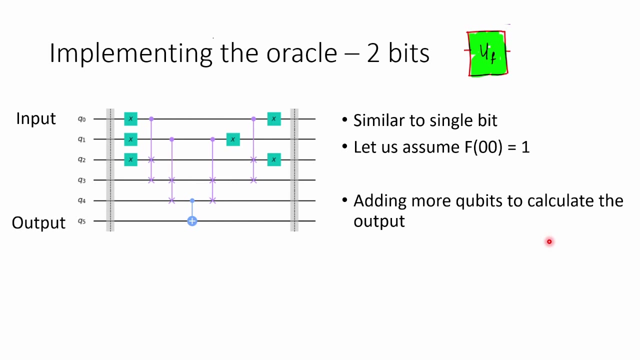 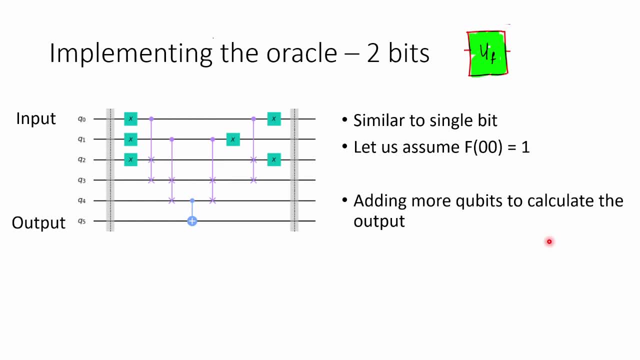 the goal is located at 0: 0, as you have seen in the previous slide. if you can implement 0 0 0, 1, 1, 0, 1, 1 is all all similar. we just have to flip the particular bit with 1. 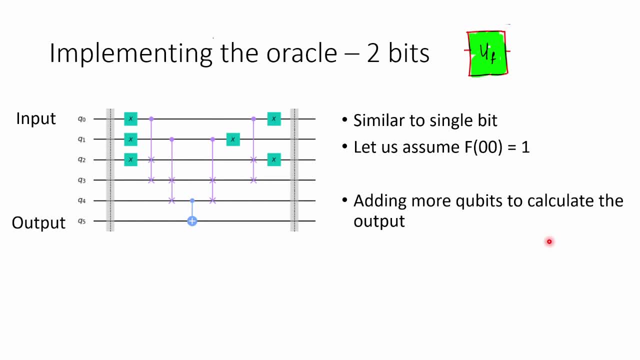 so what do we need to do? we need to add more qubits to calculate the output. exactly one more qubit to calculate the output. previously we had q0- q1, now we have q0, q1, q2. one extra bit for input. then we had two bits for answer in one bit implementation over here we have. 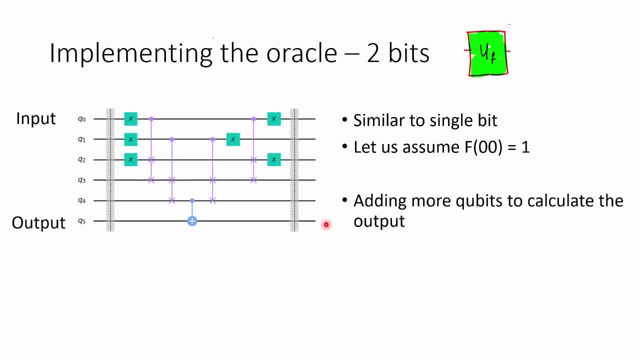 three bits to calculate the answer. so we add one extra qubit for finding the answer. how are we going to do this? if you look carefully, this part is exactly same as a single bit. say: q 0 is c swapped or anded with q2. the beginning of the. 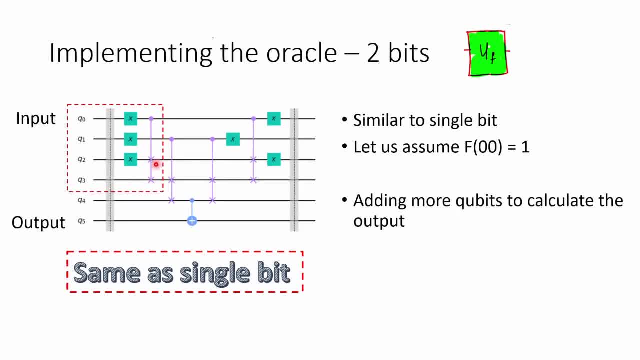 answer BIT, and then the result is store in q3. this is exactly the same as what we have seen in the previous slide. after that, what happens is we repeat the same thing, same step with q1 and the new answer, qubit q4, thinking of the next step with q1, little qubit q4. so we have a 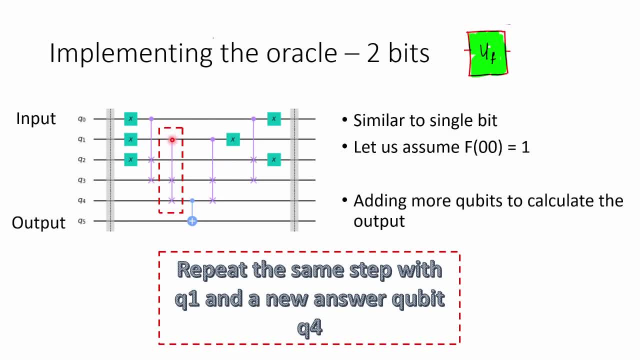 q1, now we have 1 or one. that is the new answer. the answer qubit, q4, now 1. oh, wait a minute, just let me see now. and then the new answer, which is q4. so we repeat the same thing that we did for one bit. for the second bit, q1, does the C swap or an ant with q3 and store? 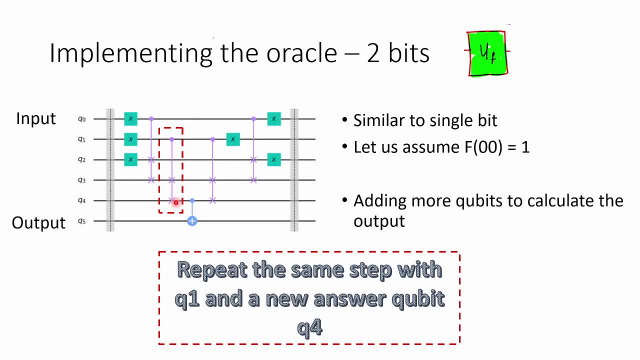 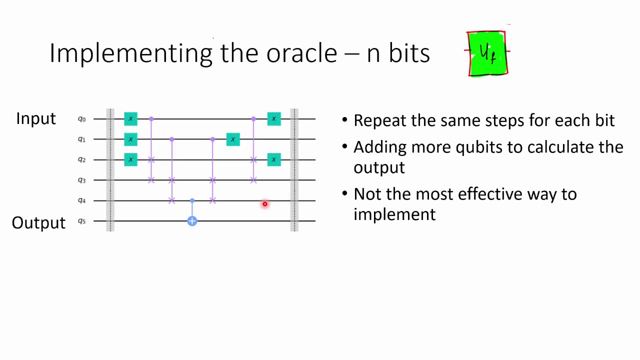 the value in q4. now, once we have q4, that will be stored in q5 and everything is reversed using the inverse gates. that is 2-bit implementation. and how can we do the n-bit implementation? you repeat the same step by adding one extra qubit for. 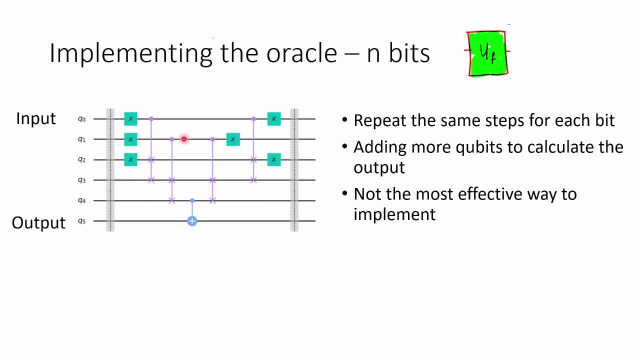 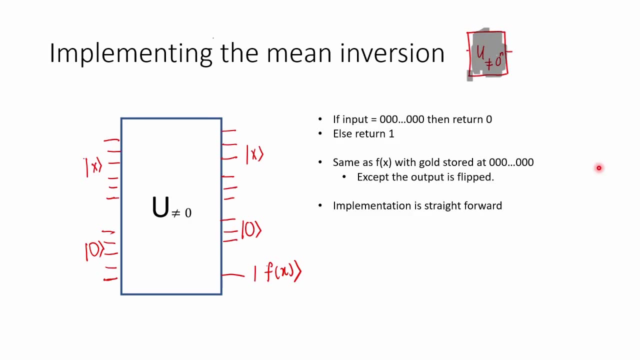 answer and just adding one more C, C, swap or ant with the new qubit and the previous answer. that's all you need to do. now you let us see how the mean inversion is implemented. so mean inversion function is looks very similar to the Oracle. so let us let me say what this? what is the 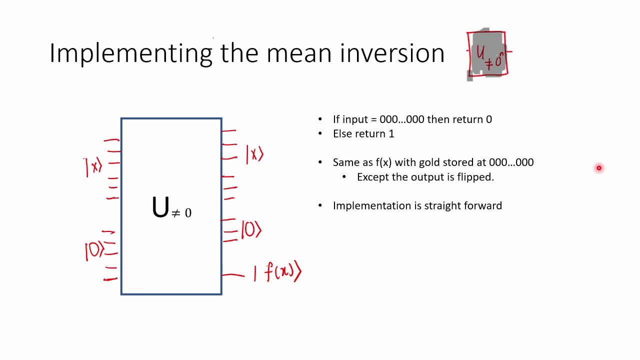 input to this function. and what is the output? it is expected very similar to the Oracle. you have an X here, an n-bit number and an F of X. right, it's not F of X, it is, we should be, the mean inversion value. the result that we are expecting here is if the input is 0- 0, so if all the input is 0. 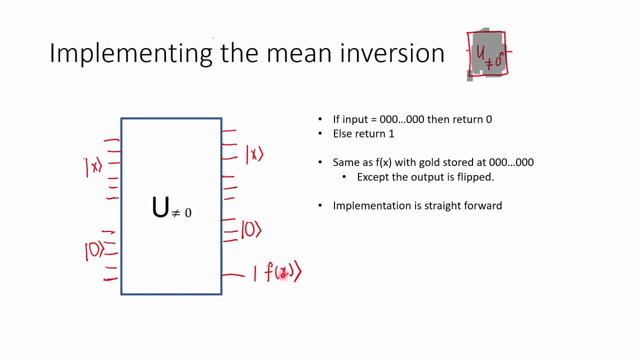 then this becomes 0, else it returns one. so when you think about it, it is like the gold is stored in zero, but the result will be just the opposite, like if it is a, the Oracle. if the result is zero, zero, zero, zero, it will be one. everything else will be zero, right. so it's very 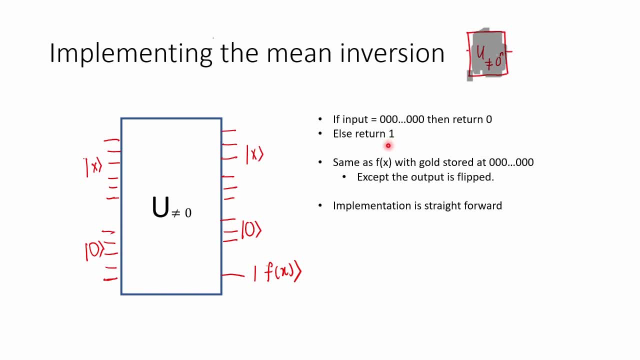 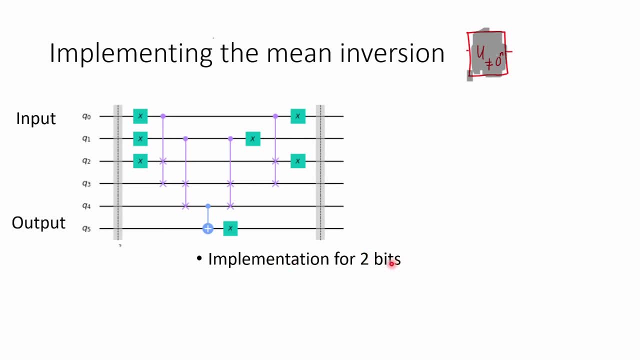 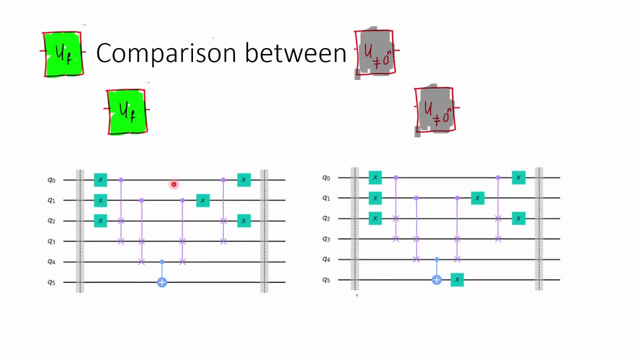 similar to oracle, just that the output is flipped right. so the implementation, therefore, is very easy for this one. this is the implementation for two bits. you may not understand the significance now, but if i compare it side by side with the oracle, you can see that it is exactly the same- the oracle. 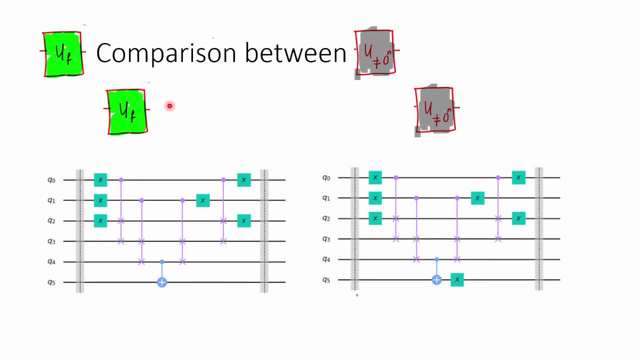 for zero, zero, f equal to zero, u of f of zero, zero. uh, i mean, the gold is hidden in zero, zero for that oracle and this one for the mean. that mean inversion is same, except for the output bit is flipped, so its output here is zero, output here will be one. the output here is one, the 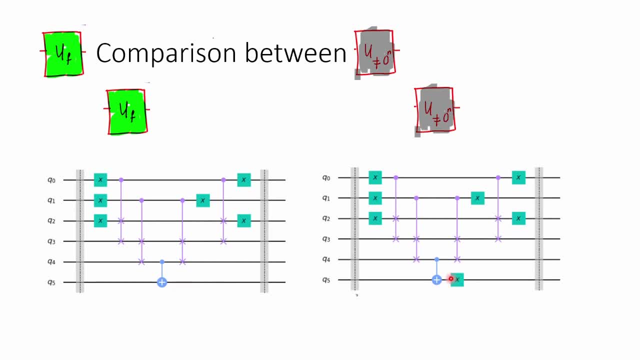 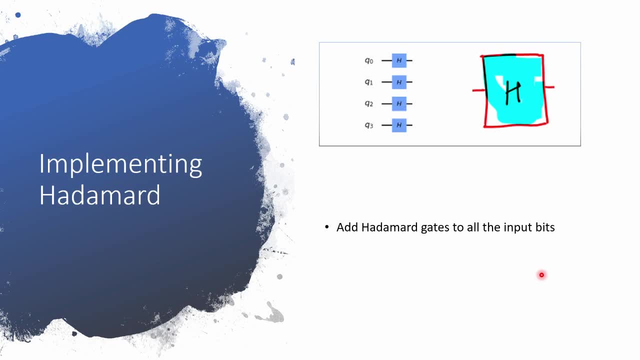 output here is equal to zero. that's the only difference for this implementation. now let us see how to implement hadamard. hadamard is a basic gate in quantum computing, so what it does is it takes a zero bit and convert it into a superposition state where the bit is both zero and 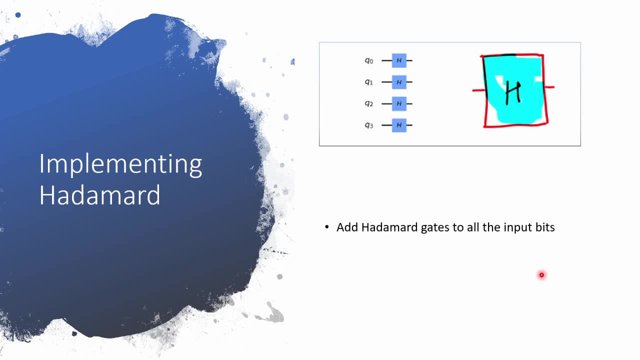 one at the same time. same with you know, if it gets one, it convert one into a superposition state where it is both zero and one at the same time, right? so we put hadamard. apply hadamard gates to all the input bits. that is what the hadamard 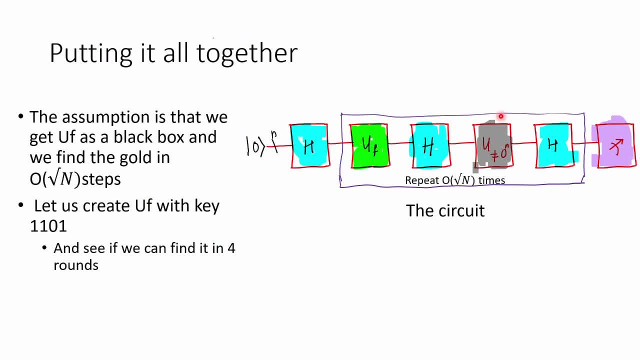 gate is. so with that we have all three components that we need to put all these things together, right? so the assumption is that we have the, the oracle uff as a black box and we find the gold, either black box in order of root and steps, right, we don't know what is inside this, of course, when 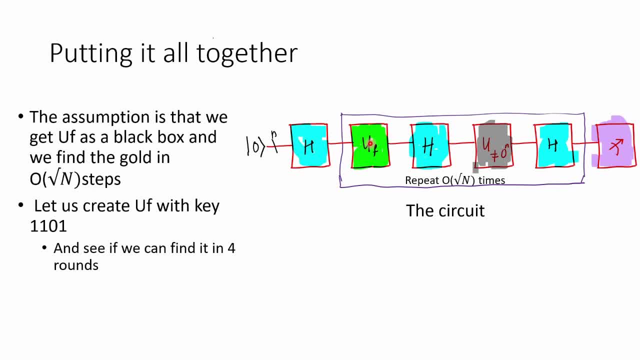 we make it be annoyed, but once we make the uff, we'll give it to someone to find that right. so so let us create a uff with key 1, 1, 0, 1. okay, so it is a 4 bit number, which means there are maximum. 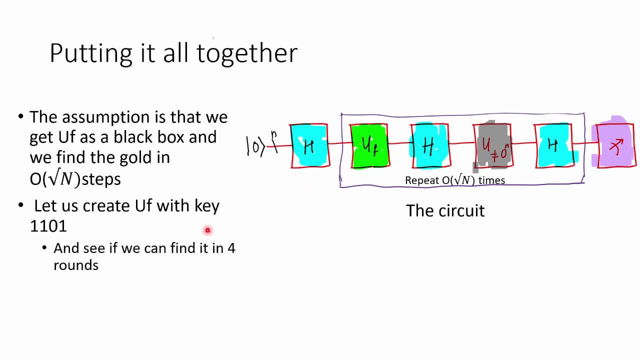 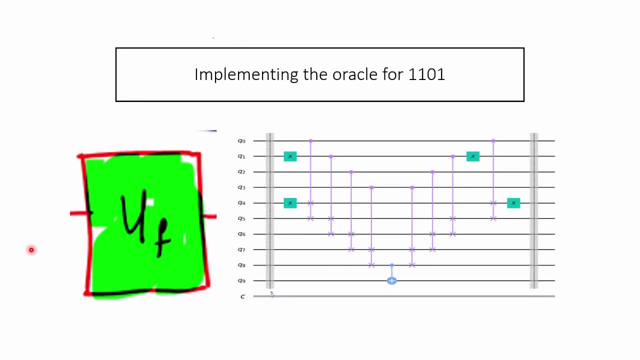 of 16 elements in that array, root of 16 is 4. let us see: if we repeat this for 4 times, we can do the magic and find 1 1 0 1 with a very high probability. so this is how the implementation of the oracle looks like for 1 1 0 1. this is very similar to the 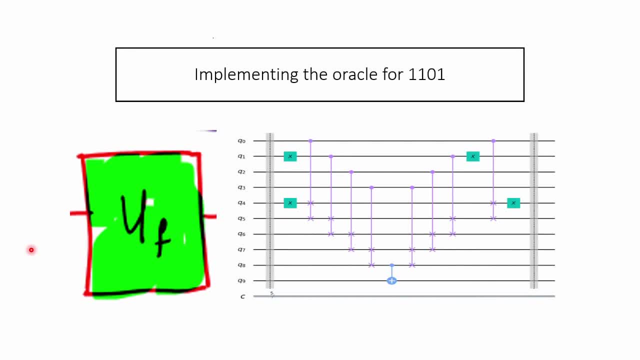 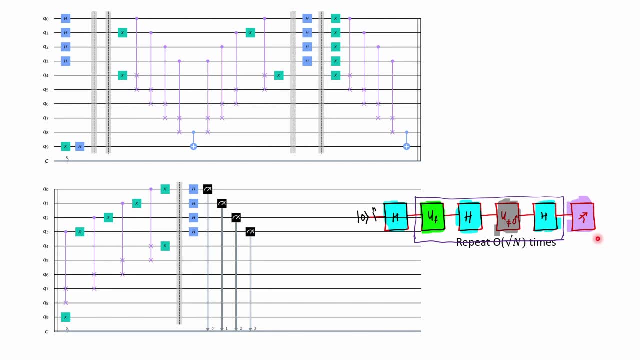 2-bit oracle implementation that you have seen, just bigger in size, and this is how the full circuit looks like, not the full circuit. this is just one iteration of the circuit. so here are the four bits: q0, q1, q2, q3. you have the hadamard gates applied. 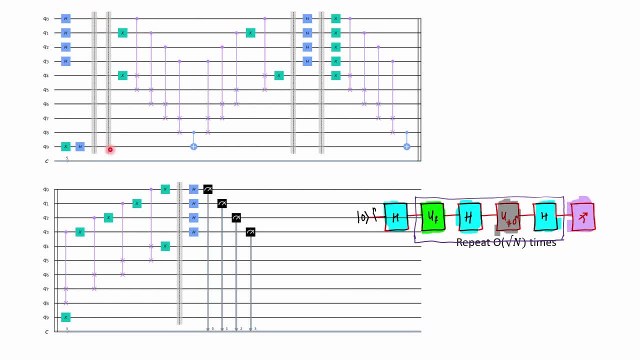 right. so this is the first period, the first part, and then this box. here is the uff. so you have the uff, you have hadamard gate, and after uff you have hadammard gate. so there is a hadamard gate. here in this small box, the input bit is applied to the hadmard gate and after: 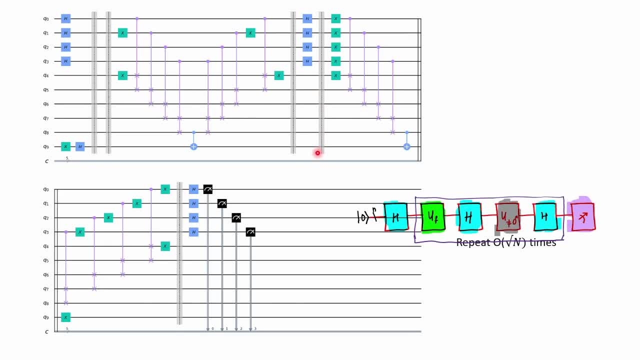 the hadider gate. what we have is is a mean inversion. so this part here, from this box until this box, is the main inversion, and after mean inversion you have the haddermard gate right. so after this, all these steps, installation part, we don't have to do that from this point all the way until this point. 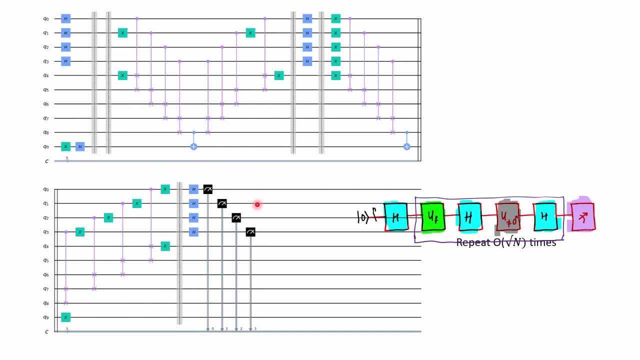 has to be repeated over and over and over. right, this is repeated over and over so that, uh, we get the correct answer. it is repeated how many times? four times. after it is repeated four times, this part is repeated four times. then we measure. we measure all the four bits: q0, q1, q2, q3.